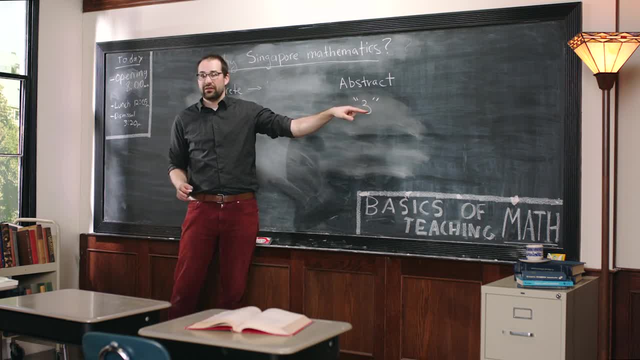 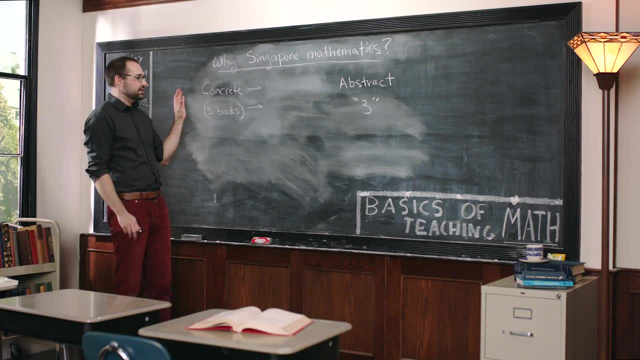 to just representing them by the number three, And I think this is a very difficult shift for students. It's hugely important. This is one of the reasons why we do teach mathematics- is it helps students think to say I'm going to take something that's a real-world problem. 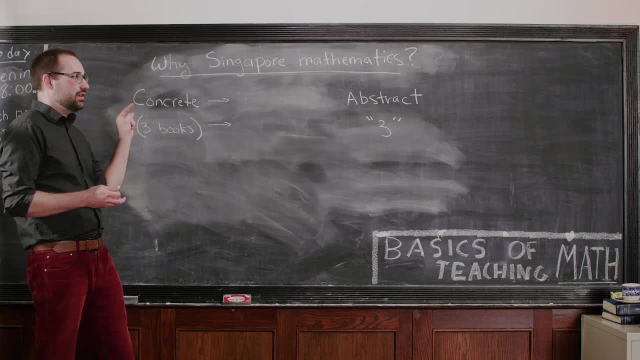 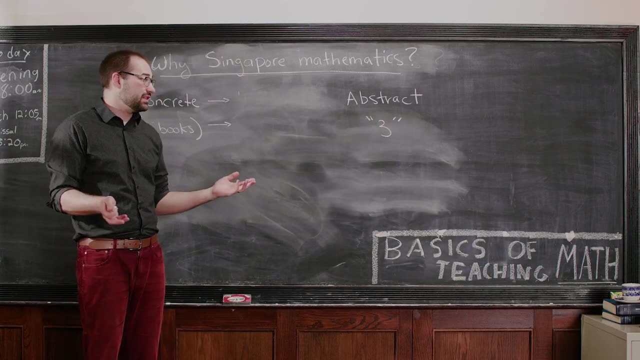 something that's in the concrete realm and I'm going to use mathematics to abstract it so that I can deal with it. And if I'm going to add three books to like three books, seven books, I don't want to have to like: put three books, get three books out, get. 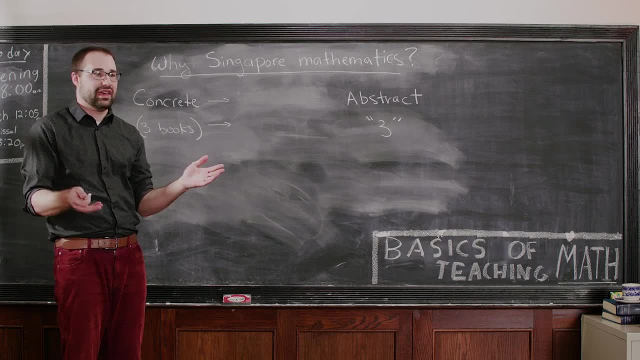 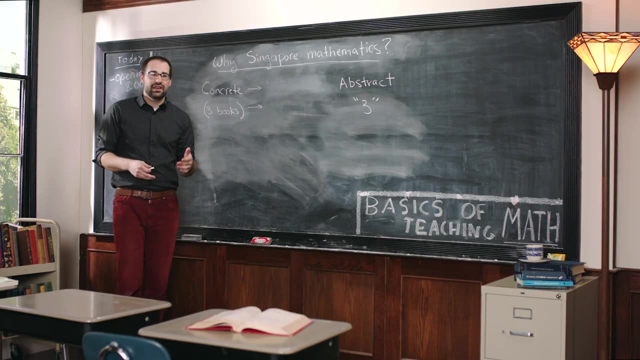 seven more books out and combine them all and then count how many books I had. What I really want to be able to do in mathematics is to take the three and add it to a seven and use the symbols. So that's why we want to teach mathematics, But the shift is actually. 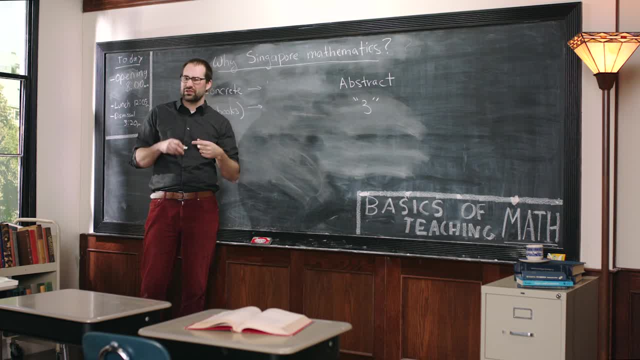 very difficult for students Abstracting something, especially if you put your kids in their first grade, second grade, third grade. it's actually a skill they don't have. This seems to adults. oh, of course we would have to do this, But it's not. It's not, It's. 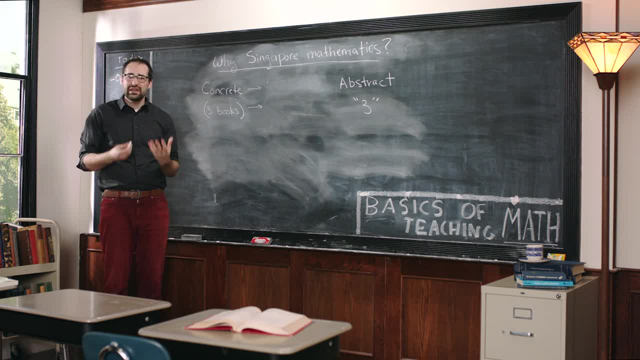 not. We would use that symbol to model that reality. But for students this is a struggle And this is a big leap over into the abstract. So the brilliance of Singapore mathematics lies in the ability to take something to help students make this shift. So to go from the 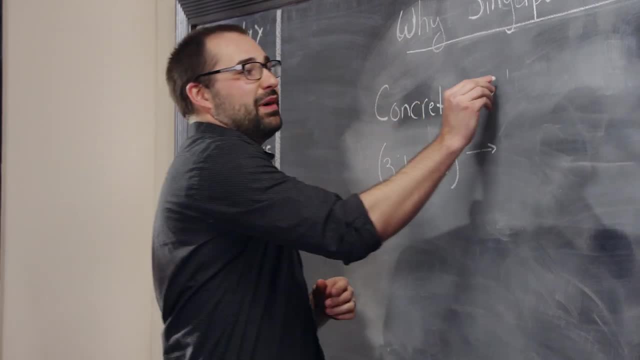 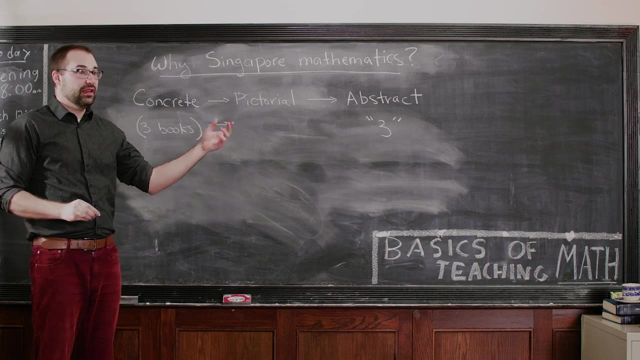 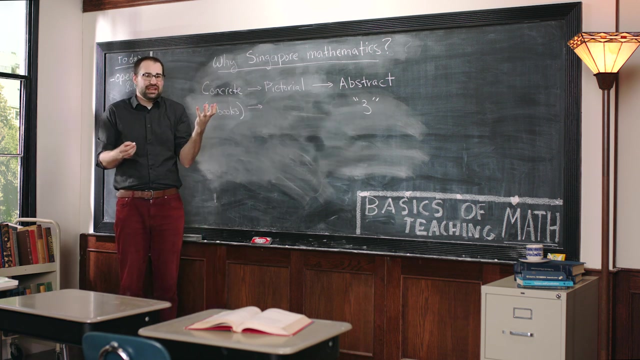 concrete to the abstract. what we do is we have them pass through the pictorial That we use this as something that is. This is an easy way to shift from the concrete to the abstract. It's somewhere in the middle. It's not concrete, It's not abstract, But it participates in them a little bit of both. 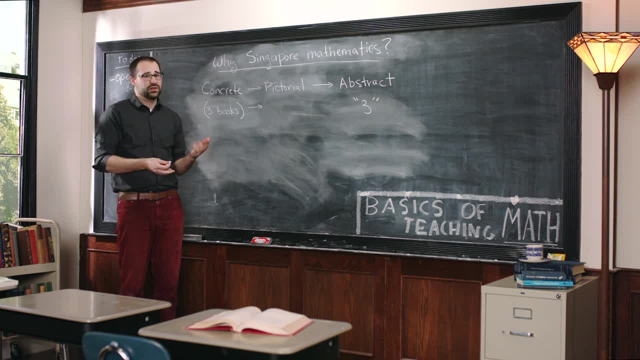 And it's universal. Everyone's actually able to draw pictures, And that's actually the reason why Singapore math got invented in the first place is when the country of Singapore shifted its language of instruction to English. students had a hard time grappling with this. 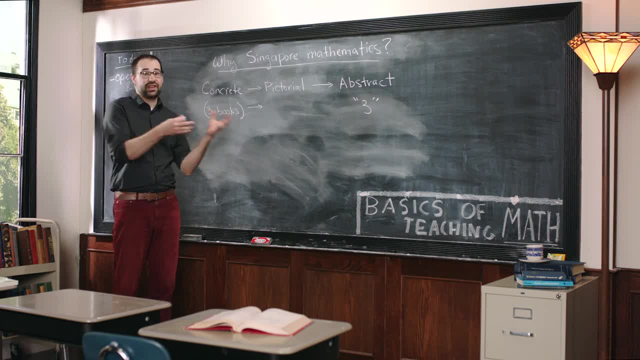 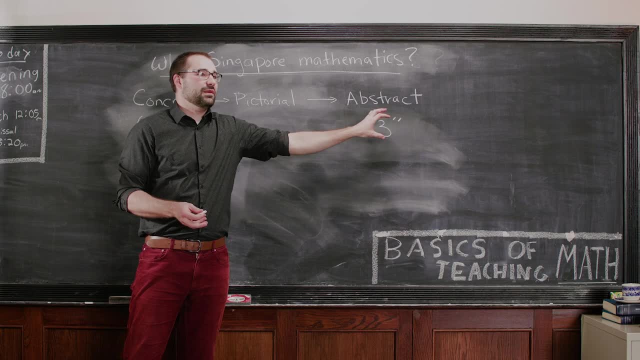 new language. And so what they did was they inserted a bunch of pictures into the pictures, Into their mathematics program in order to help students make sense of it. Think of mathematics as students learning the language of mathematics. These pictures really end up helping, So what? 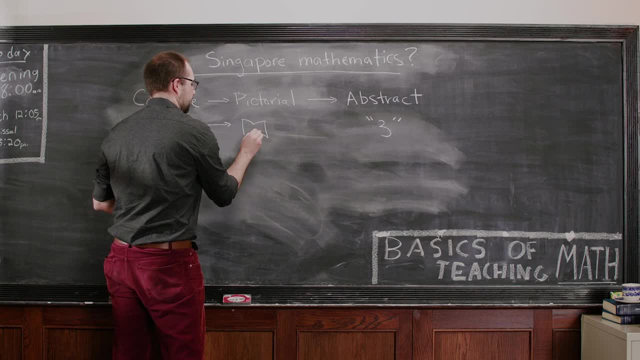 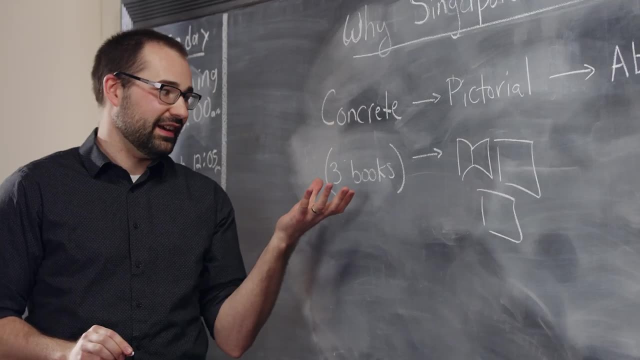 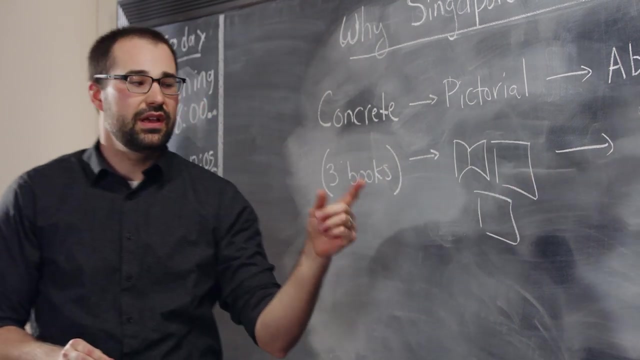 I could do is draw something. That's not a very good book, But you get what I'm saying here. if I draw, This is not really. It's not concrete, They're not physical things I can hold, They're not abstract in that it's not just a symbol, But they're a way to make. 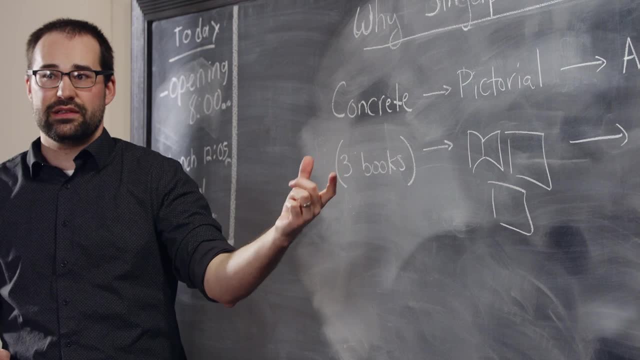 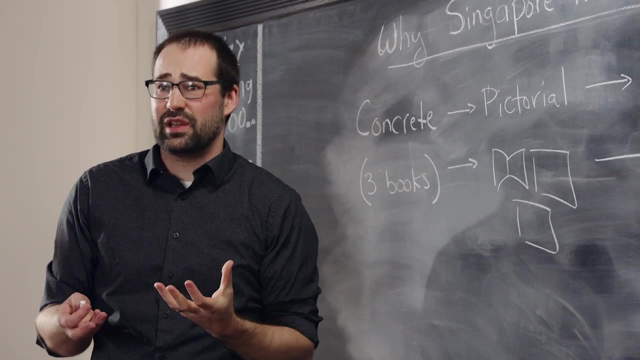 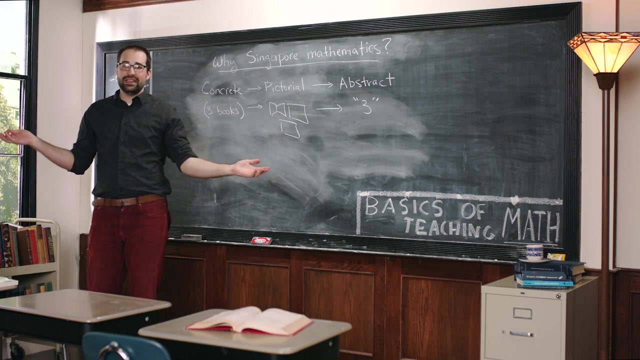 a transition here From the concrete to the abstract, And you might be thinking: well, I don't need three books here to make that transition right. So how does this actually play out in a real problem here? Pretend if I have a concrete problem. Maybe I have 19 students and then 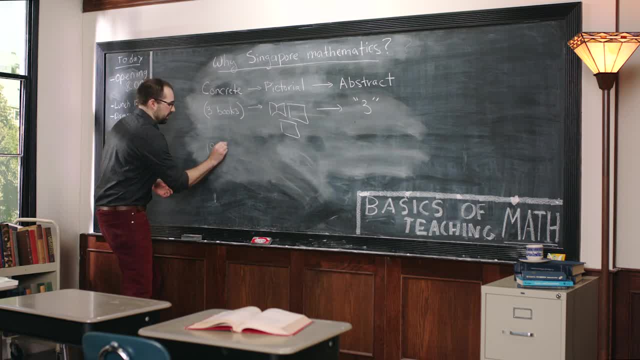 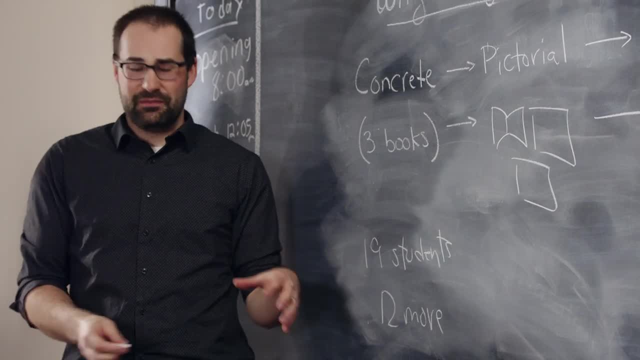 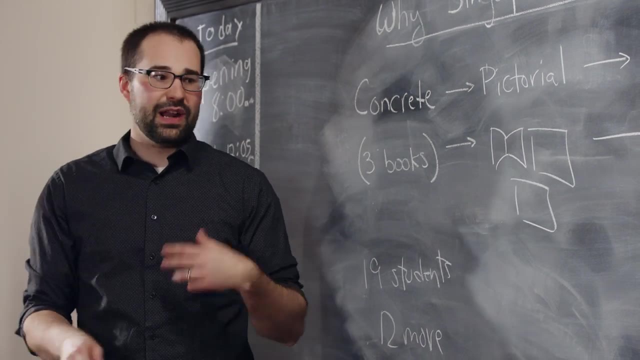 I get 12 more. I'm not going to have the concrete students up here, But you'd have to imagine them physically standing here with me And I want to know how many students I have in total And what I want students to be able. 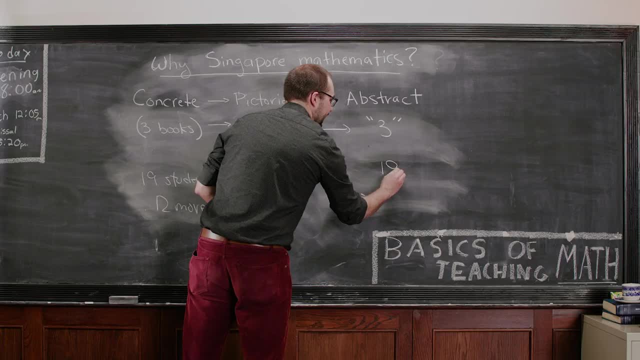 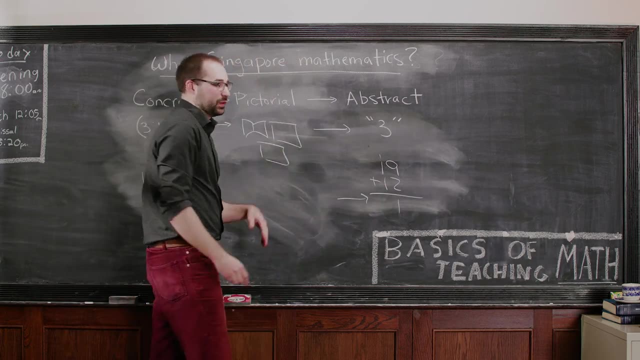 to do is over here in the abstract realm, where I have 19 plus 12. And I take my 9 plus 2 is 11. And 1 plus 1 plus 1 is 3. And I want them to be able to get my answer of 31 in. 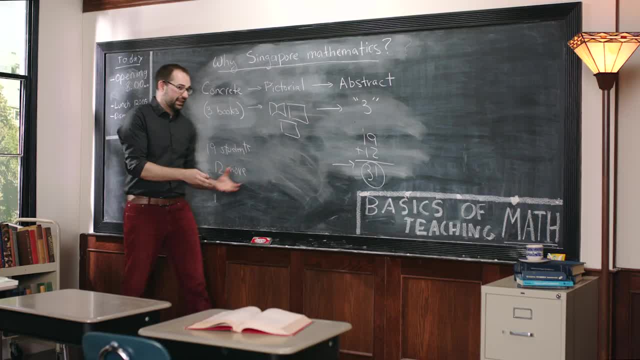 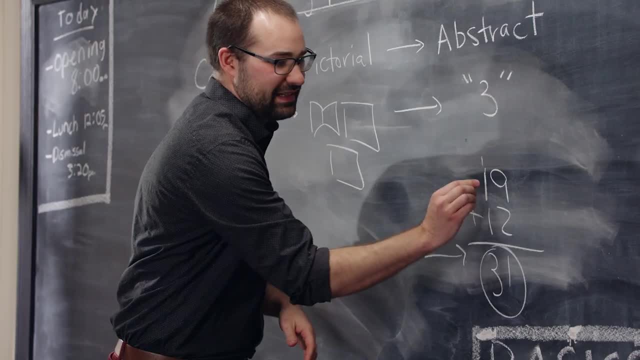 the abstract, But this is a big leap for students. They can count over here. They've got to do this symbol jigger around the relationships here. You're taking these symbols, You're moving them all around And this is very difficult, right? This is actually. this seems. 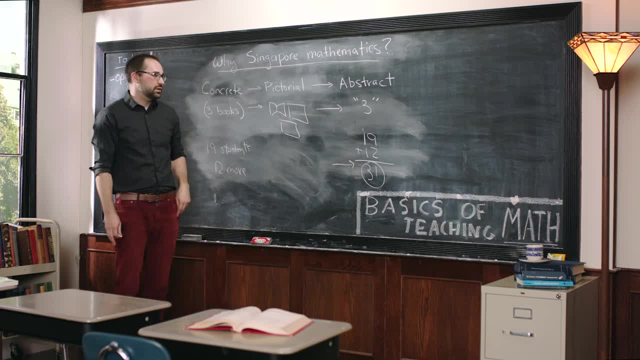 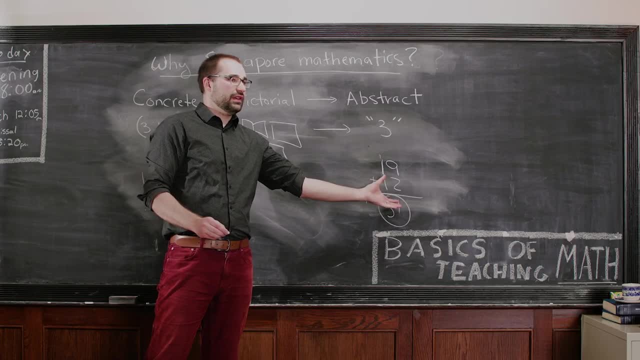 very natural to us as adults, But it's actually very difficult for students here, And so how do I get a student to progress from over here, where they're just counting, to be able to do an operation like this? Well, I want to figure out what picture I can draw, right. 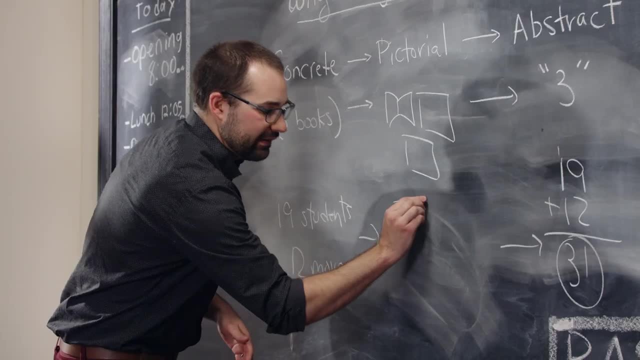 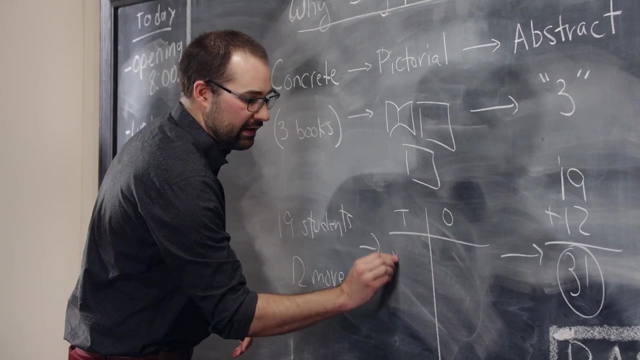 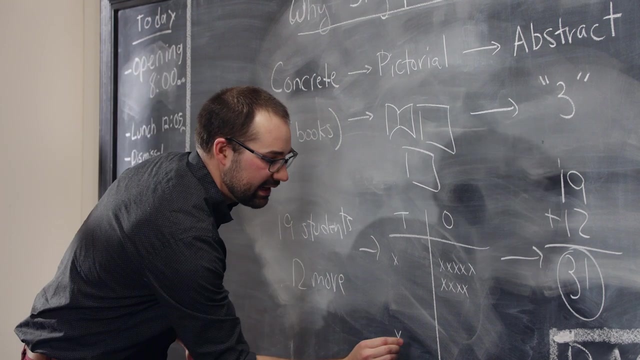 And so what we do is we draw a picture like this, where I can say, OK, I have tens and I have ones here, And 19 students is made up of 110. And 9 ones, And 12 students is made up of 110 and 2 ones, And what I want to do is push these two things.